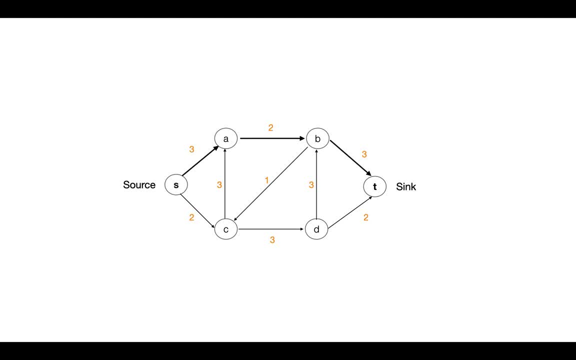 able to pass two units from this edge BT as well. So the thing is, the amount of fluid, or you can term it flow, in this path or in any path from source to sink is limited by the bottleneck capacity of that path. In this path that we 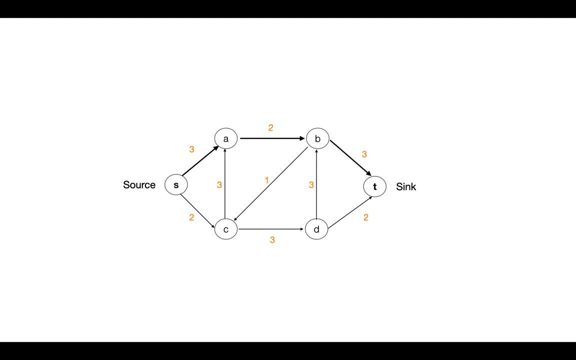 discussed that we have taken from source to sink. the bottleneck capacity is two, So we cannot transfer more than that. And the bottleneck capacity is two, So we cannot transfer more than that through this path. so this was the first path that we selected. if we are selecting this path, that means 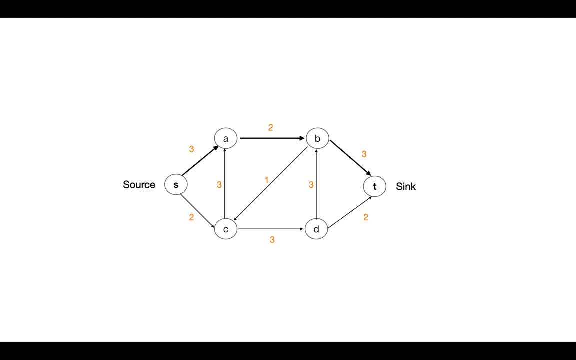 we are passing two units of water through this path towards the same t. so now we're gonna write this flow across the respective edge along with the capacity. so we, if you see this edge sa, the capacity of this edge is three and the flow across it the current flow across it. 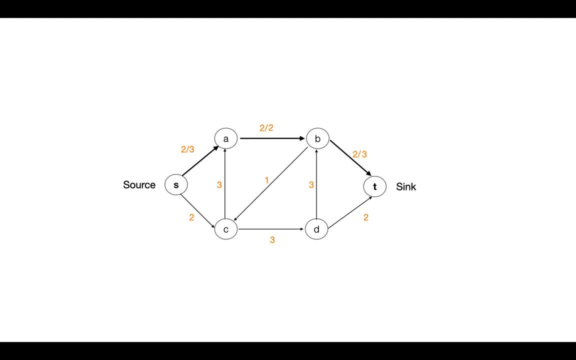 is two, so there's still one unit of water that can be sent through this edge sa and this remaining amount or this remaining space for one unit. we term it as residual capacity. so residual capacity for s? a is one and for this edge ab is zero. as 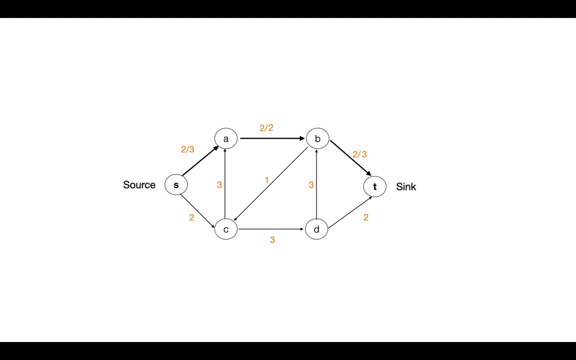 the current flow is two and the capacity of this edge ab is also two, and now this edge bt, the capacity is three and the flow is two, so it can allow one more unit of water through it. so this was one path. we can choose more. there's another path right here. it is s. 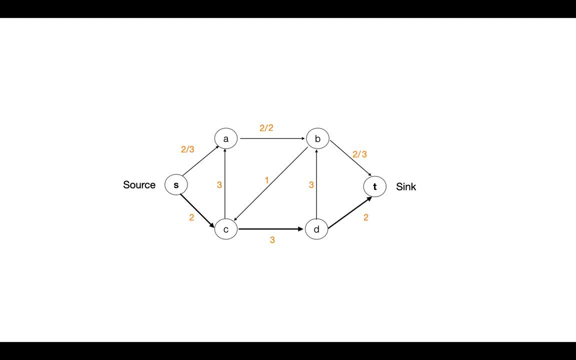 to c, c to d and d to t. again, the minimum capacity of this path, or what we call the bottleneck capacity, is two, so this path can also take two units of water to the sink. so we chose two paths: s to a, a to b, b to t and the second one s to c. 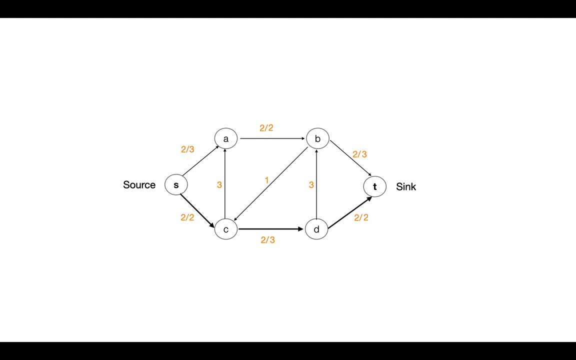 c to d and d to d. so we are getting two units to sink through the first path and two more units through the second path. that makes a total of four units to the sink. but is this the maximum that we can get to the sink? yes, this is the maximum flow that we can achieve in this network. 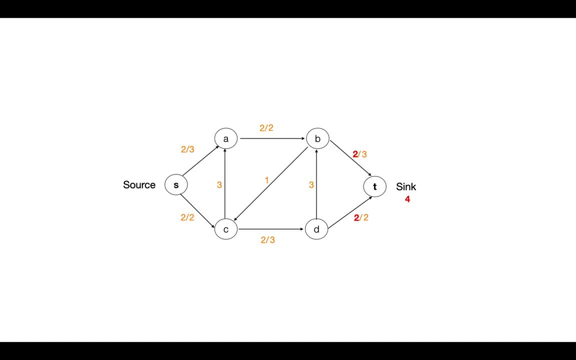 so this looks quite straight, right, but just wait for a minute. let's reset this graph back to the original network, where we don't have any flow going through any of the edges. now let's say we pick this graph and we are getting two units of water through this path. 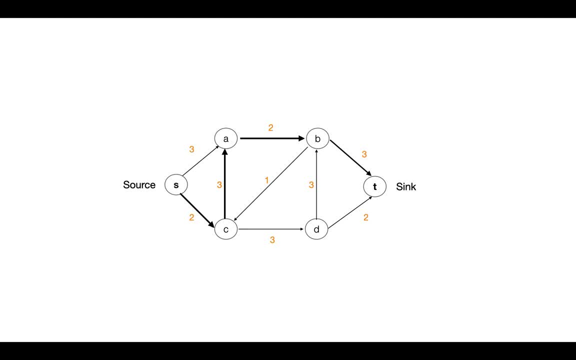 so we have two units of water through this path. so we have two units of water through this path. so we have two units of water through this path. or let's say, our algorithm finds this path first and traverse it first. so from source to c, c to a, a to b and then b to sink, i can pick this one right, because this is a. 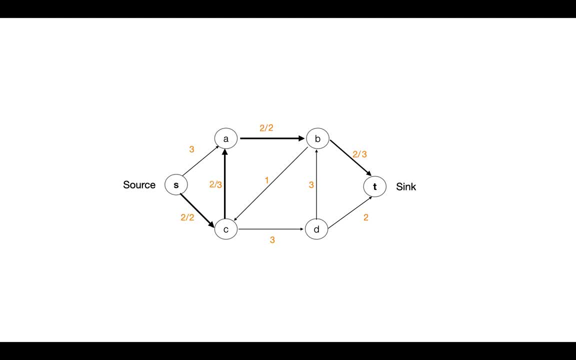 valid path too. so if i go like this, the bottleneck is that we have two units of water from source to sink, so this path needed two units from source to sink. now let's find more paths so we increase the flow. we are getting at the sink right. so is there any path? 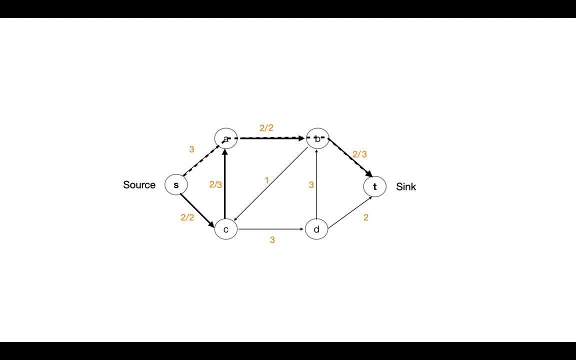 what if we try to go like this, from s to a, a to b and then b to t? so see here, this edge a, b is already filled up to its capacity. so if we try to go from a, from s to a, then we won't be able to. 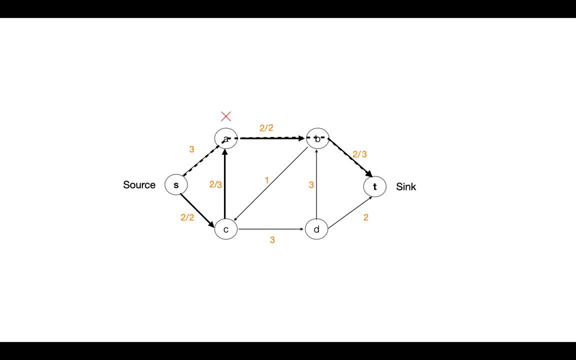 carry it forward to the next edge. so we will be blocked right at this edge, right at this vertex a now, if we try to find some other path, which can only be possible if we go from s to c, but again see this edge, s to c. the capacity of this edge is two and the current flow is also two. there's. 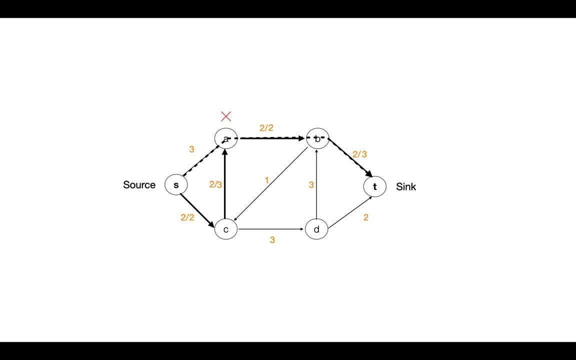 no space left for more water. so we can't push more water from source to c. again we are blocked here. so if we first pick this path- s to c, c to a, a to b and b to t- the max flow- i should not term it max flow- the flow. 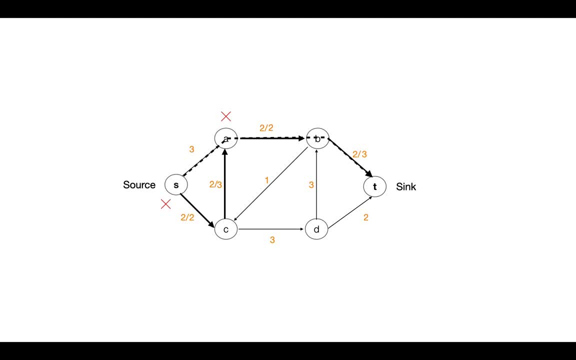 that we are getting in this network from source to sing is two, but this is not the max possible flow- three days. it's only one question, though. these two buttons are two and this needs the maximum lowerน the network. We saw it a few minutes ago that the max possible flow through this network is 4.. 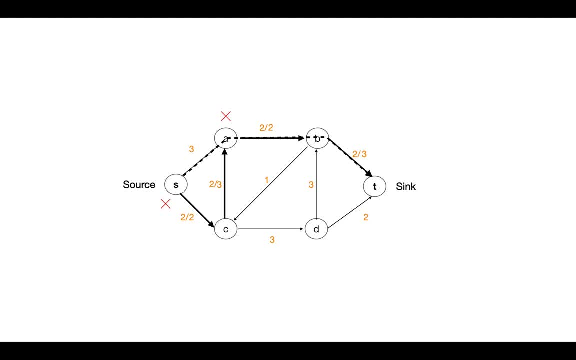 So finding a forward path from source to sink in this original graph may not always work. And here comes the concept of residual graphs. Ford Fulkerson worked with residual graphs to find the paths from source to sink rather than finding paths directly in original network. But how we gonna get benefited by residual graph? 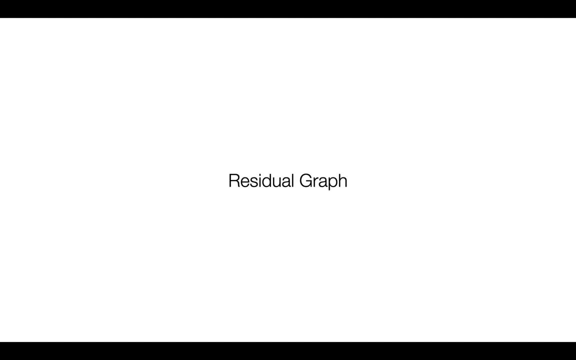 You'll get in a minute. Residual graph, as its name implies, is something that has residual capacities. okay, So to create a residual graph, there are two kinds of edges that we draw: Edge with its residual capacity and edge with its shrinking capacity. So let's say, this is the network whose residual graph we are going to draw here. 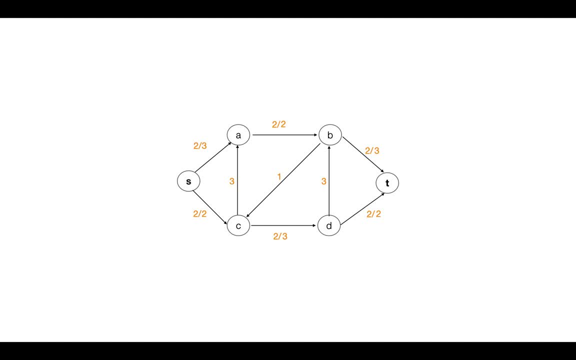 So this network is the one we got when we were getting a max flow of 4, by selecting two paths, one from s to a, a to b, b to t and the other one from s to c, c to d, d to t, right. So, 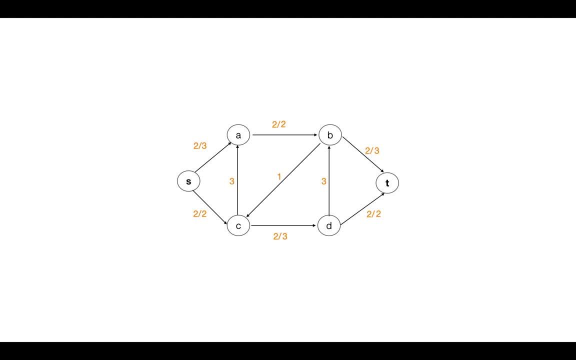 see this graph. to draw its residual graph: first, we take all the vertices that we have in this original graph. Now let's draw the edges. Let's start with S. A See in original graph. the flow in this edge is two and the capacity is three. So this edge is capable of passing one more unit of water from. 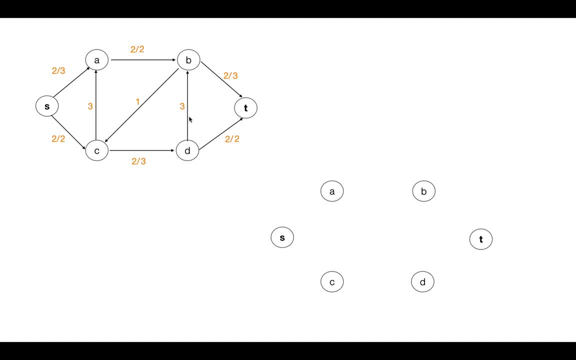 s to a, So its residual capacity is one. Now comes shrinking capacity. This edge, you know, is having two units flowing through it, through it. but this current flow can also be shranked back to zero if required. so this vertex, a, can say no to the source for this flow, or for a part. 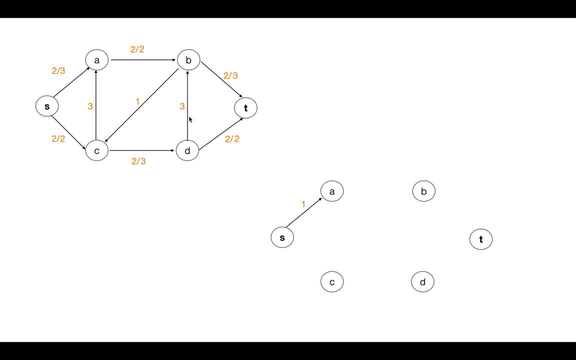 of this flow. it's a possibility. so if those units can add more value to some other path in network, we can undo the flow. so we can undo two units from a to s or we can say the flow can be shranked back from two to zero. this is the way. 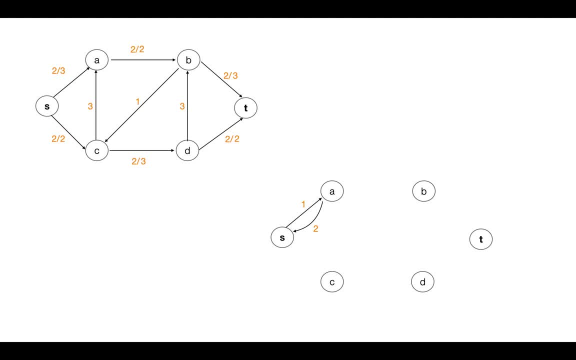 how we show it two units back to source from a. so residual graph comes with the concept of shrinking the flow through edges, which indeed is important. now let's take the next set of vertices: a- B. the current flow across a B edge a B is 2 and the capacity of this edge a B is also 2. so the residual capacity, or 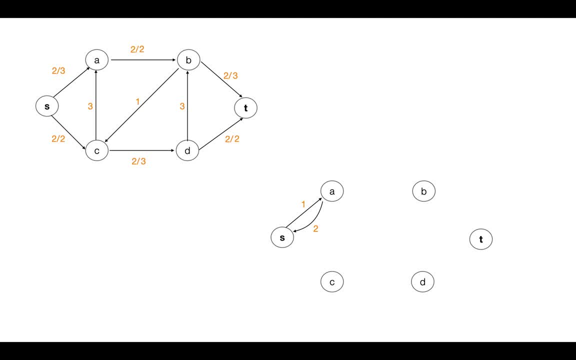 remaining capacity is 0. we have no space to increase the flow further. that's why no forward edge. we're not going to draw any forward edge. we can only undo two units from B to it. now let's take next set, which is B T. current flow across B T. 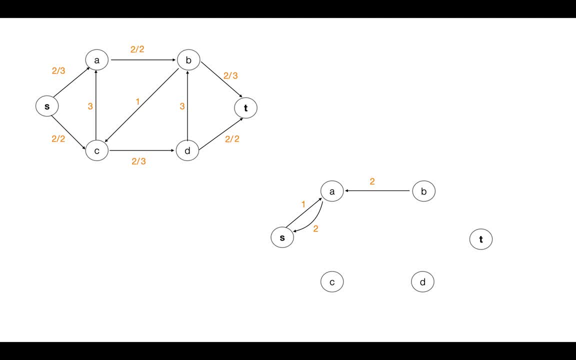 is 2, but capacity is 3, so remaining or residual capacity is 1, so it can pass through one more unit and it can undo its current flow by 2. now let's take S C. it's not having any residual capacity, it can only undo two units flowing. 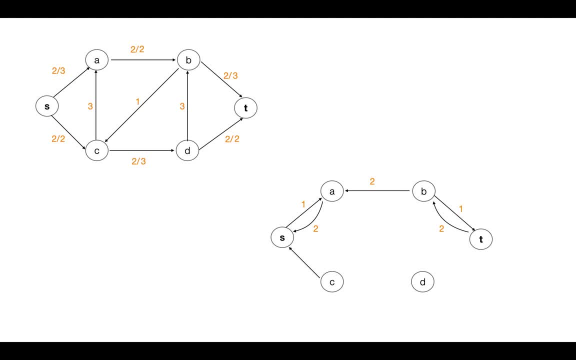 through it, so only a backward edge. next is CD. we can increase current flow by 1 and we can shrink it by 2. so forward edge with 1 and a backward edge with 2. now this one, D T, no residual capacity, but we can shrink it by 2. now the remaining three edges, the 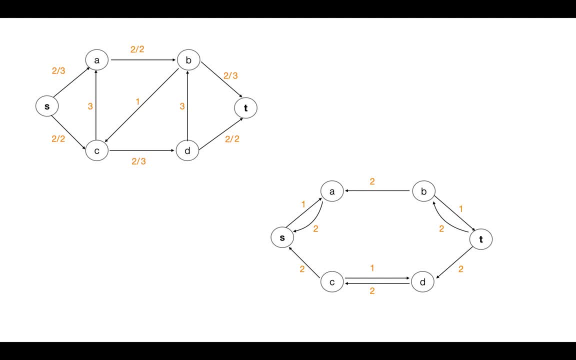 capacity and residual capacity. both are same for these edges as a current is zero, but we can shrink it by two. now, the remaining three edges: the capacity and residual capacity. both are same for these edges as the current is 0. capacity: both are same for these edges as the current is zero. 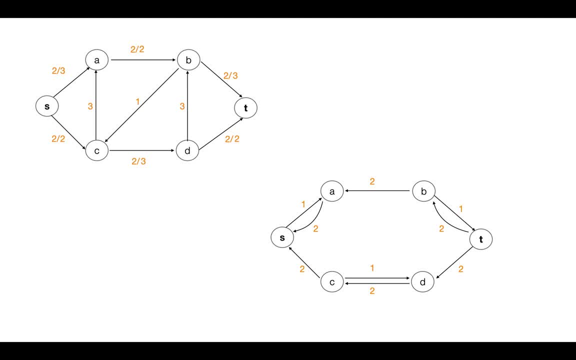 UNG girded by current flow for the first and the total current flow became 0. just to enhance current flow again 1. we can hit. attention, we use cd. we have the is zero. current flow is zero for all of them, so they can allow water equal to their capacities. 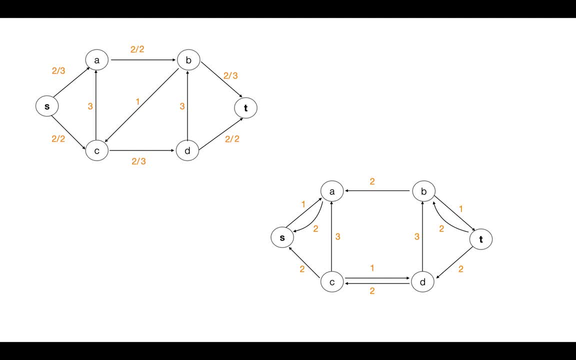 so we're gonna draw them just like they are in the original graph. so this is the residual graph. after drawing this residual graph now we can shift back to the greedy way, where we now look for the forward paths from source to sink. it does not matter whether the edge, the path is covering. 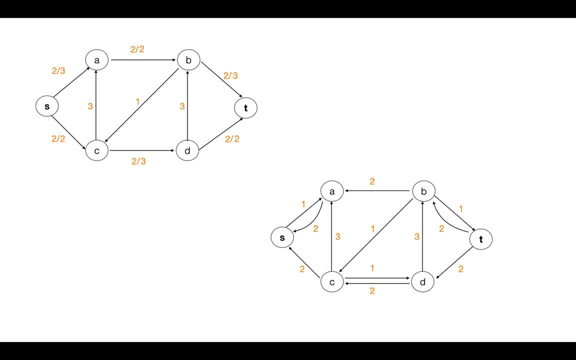 is one for residual capacity or for shrinking capacity, but it must contribute to make a complete forward path from source to sink and we call this path an augmenting path. so see this residual graph. do we have any augmenting path from source to sink? consider only forward paths. 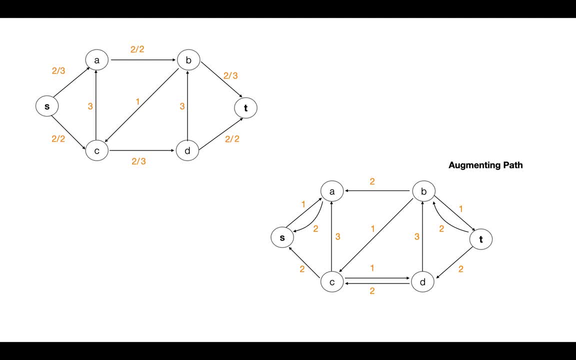 we can't include edges going backwards. okay, you'll find no forward or augmenting path from source to sink, which means the current flow through the complete network is already at max. now let's compare it with the second case, where the path we selected was s to c, c to a, a to b and b to t. so 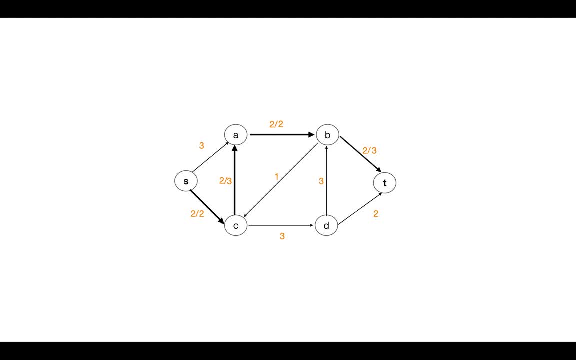 let's draw the residual graph for this case as well, just to make the concepts clear. so here let's take the vertices. and now let's start with s a. the capacity is three, and currently there's no flow across this edge. so the residual capacity is also three. and now the next edge. 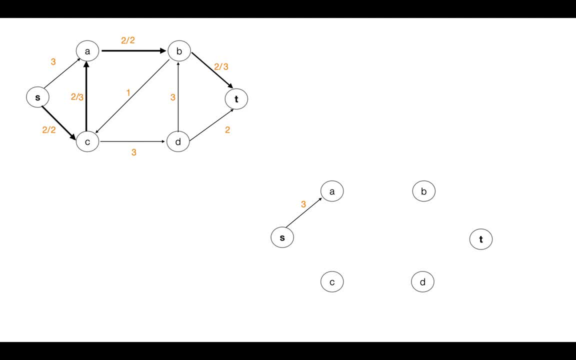 next set of vertices is a- b, where we are having capacity equal to two and the residual capacity is zero as it is already filled by two units of water. so we can only undo two units from b to d. a Now bt, where there is space for one more unit of water from b to t and we can undo two units from. 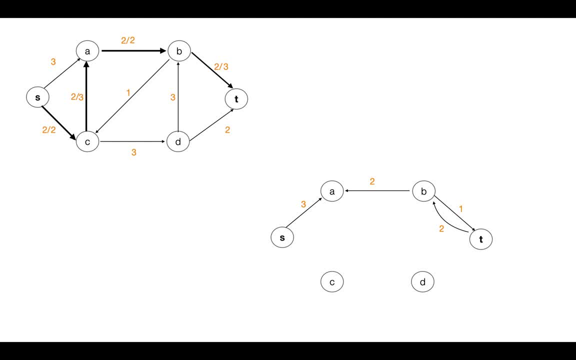 t to b. Now. next is sc, where we have no space for more water, so we can only undo two units. Now cd, where there is no flow. currently there's no flow, so the residual capacity is equal to the capacity, and the same is true for dt. the residual capacity is two. And now next edge, ca: see this edge. 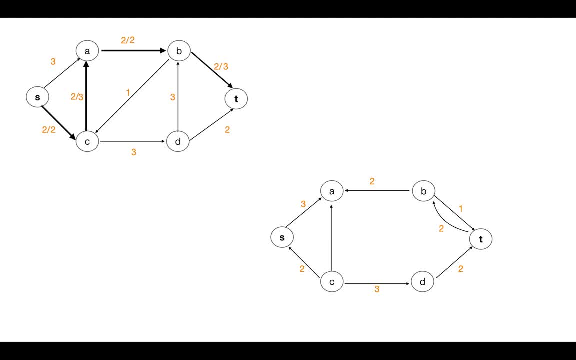 there is space for one more unit from c to a. so residual capacity is one and we can shrink back the flow by two. Now the other two edges: they're not used, there's no flow across them, so let's draw them as they are. So this is the residual graph that we're getting. 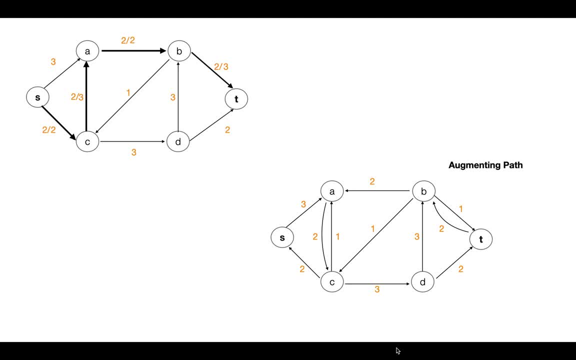 Now again, look for the fourth path, or you can say for the augmenting path. There is one from s to a, a to c, c to d, d to b and b to t. This path is the proof that we're not getting the max flow at the. 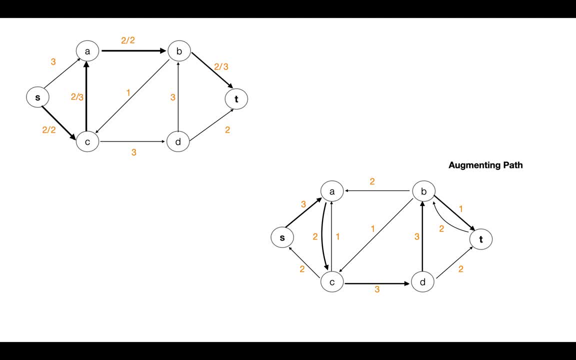 sink. yet There are possibilities to increase the flow at sink. So, as we got this path, now let's look for the bottleneck capacity. Bottleneck capacity for this path is one we have it with edge bt right, so we're gonna increase the flow by one in this path. Now look at the original network. this is the path in this sa is. 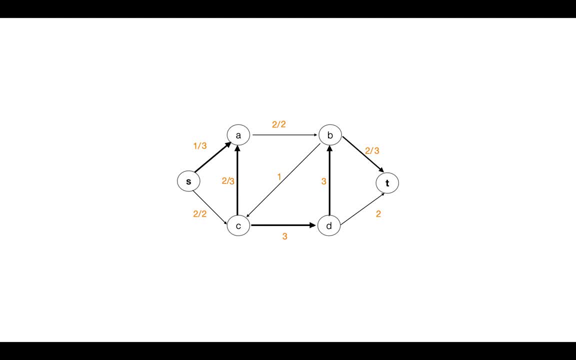 going to have a flow of one. and now comes ac. it's a backward edge, and the edge that we selected in the residual graph was meant for shrinking the current flow, right? so here we're going to shrink the current flow by one. so actually we're going to eliminate one from the current flow. 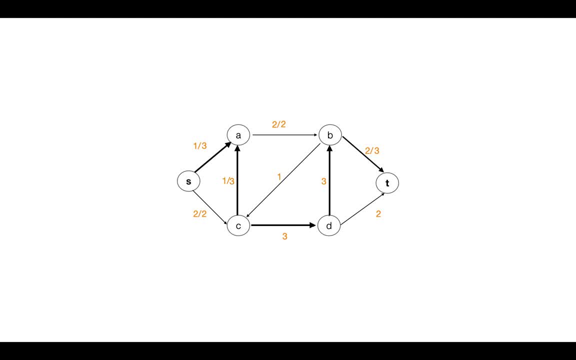 That's why now the flow through this edge will be reduced to one from two. Now let's fill one in cd, one in bd and bd as well. so with this, bd is now completely filled. so again, have a look at the updated residual graph. This is the updated residual graph. so 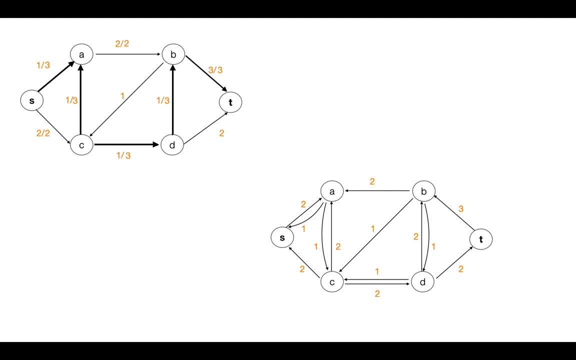 let's see again if we still have any augmenting edge, augmenting path. so yes, we do have. it's from s to a, a to c to d, C to D and D to T. so let's increase the flow in original network now, see here: 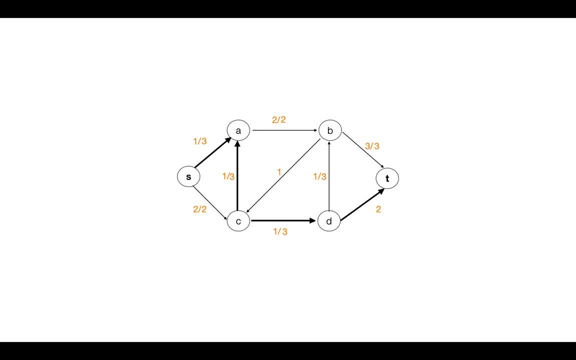 the two units that are reaching at C from source are getting distributed among CA and CD. but after we increase the flow in this path, in this augmenting path that we selected, what we're gonna get, let's see so as a: we're currently having flow of one, now it will be having a flow of two units and now AC, which is 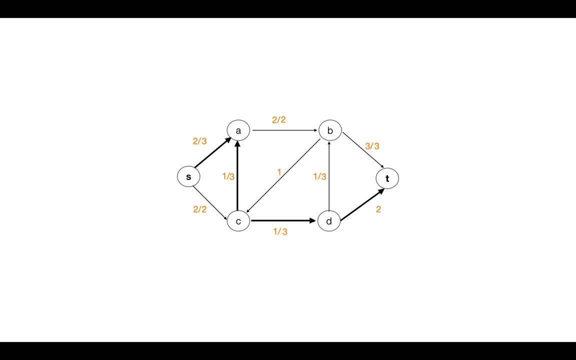 a backward edge. so again, we're gonna eliminate one from this edge. and now C D- here again we're going to increase the flow by one, and D T, where the flow, current flow, will be 1. so this is the path and this is the current flow across. 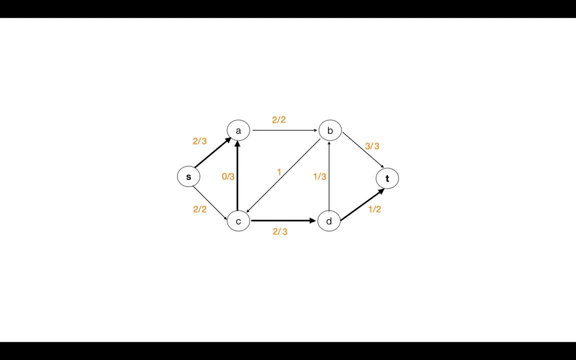 this path. now see this edge S C. here we are getting P and D C two units. These two units were previously getting distributed among CA and CD. Now CD is getting both the units. Remember I said earlier that we reduce the flow from one edge to adjust it to some other edge. That's what is happening. 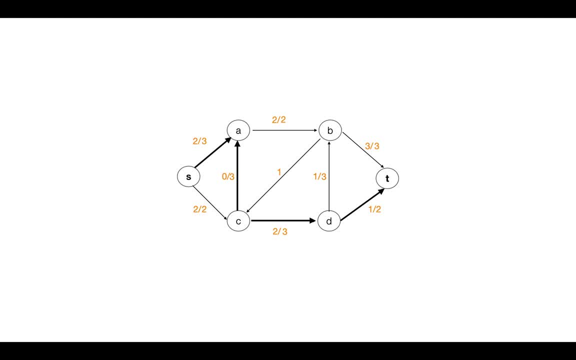 here, If two units reach to C, they must leave C towards the other vertices, and that's also what the residual graph takes care of, and that's what shrinking the flow is all about. So, in residual graph, no matter what the path you choose, 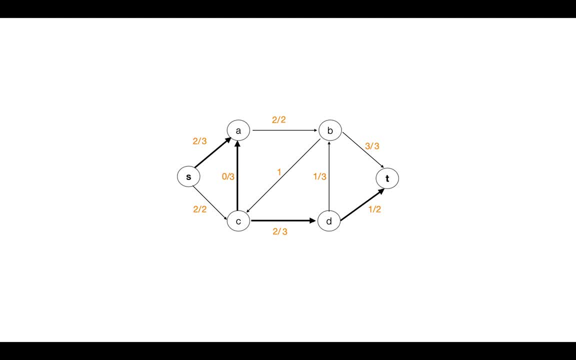 it won't block other existing paths. because here we are having the concept of shrinking the already running flow, so now we are having 4 as the flow at the sink which is in did E maximum flow. so now, if we create the updated residual network for this network we won't find. 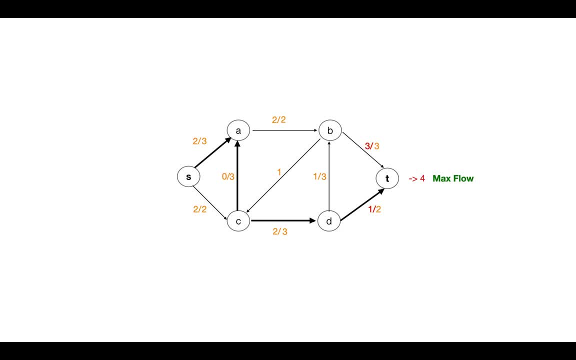 any augmenting path. so this was the core part of ford fulkerson. now let's see how we actually gonna implement this. we are not going to move back and forth between the original network and residual network. instead, from the beginning we only gonna stick to the residual graph. 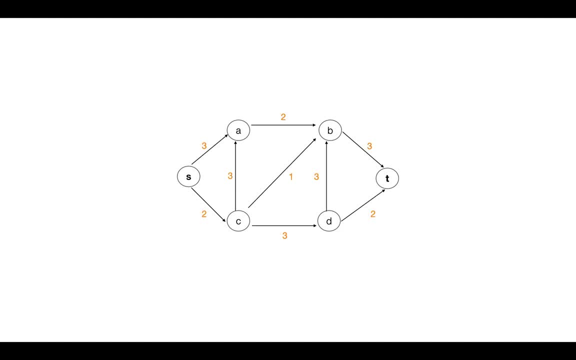 so this is the original network. now we're gonna convert it to residual graph and it's gonna be very easy as initially there will be no flow in the network. that's why residual capacity for all the edges will be equal to the actual capacity of the edges and again, as there's no flow in, 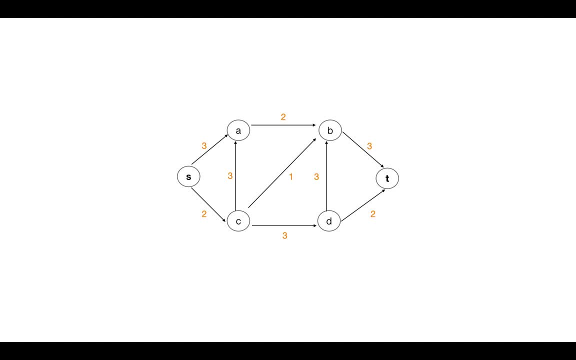 the network. we cannot undo anything right, so the shrinking capacities will be zero for all the edges. so this is the residual graph. this is the structure or graph with which we are going to start our implementation, and now we're gonna start from source to reach to the sink. basically, we are 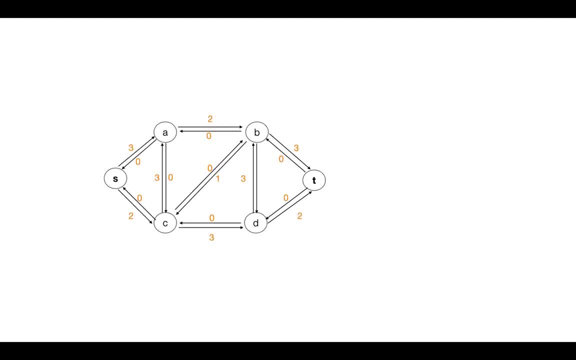 going to find out the augmenting path, and for that we're gonna need a map kind of structure- and we're gonna call it parent mapping- where we can store key values. basically, this parent mapping is the one which is gonna help us in constructing the augmenting path. and now comes how we're gonna go over these vertices, or how we're 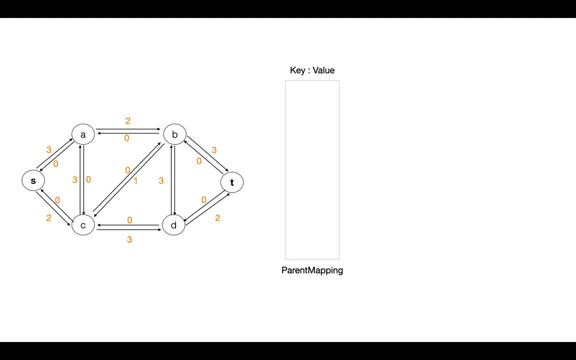 gonna traverse this network. so we can either go with DFS or we can go with BFS. it's up to us. so here we're gonna go with BFS. so for that we will be needing a queue. we gonna push current vertex in this queue and we're gonna take a visited set. it's gonna keep track of all the visited. 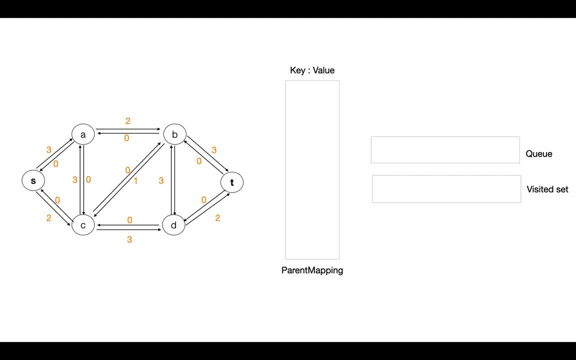 set while searching for the augmenting path in the network, so that we don't include the same vertex again in the path. okay, so let's start with s. let's add s in this queue and to the visited set as well, as we're visiting it. and now from here, loop starts. until the queue is filled, we pull items. 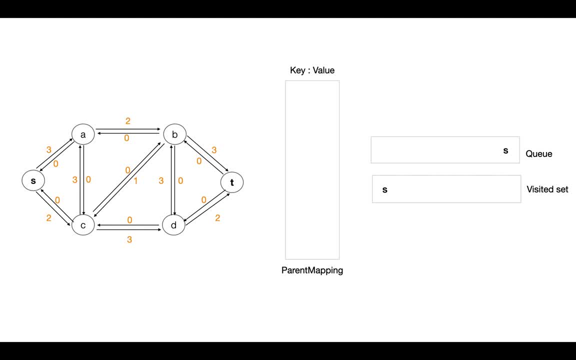 from the queue. or you can say we pull vertices from the queue, one after the other, and we start finding the forward edges from that vertex in the network till we reach to the sink. okay, so there are two things to be taken care of while selecting the edges: first, as the edge must be having value greater than zero. and the second constraint is: 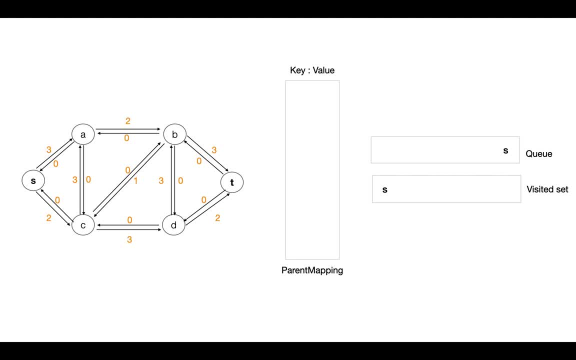 that the edge must not be already visited, so it must not be already there in the visited set. that's just. it's going to lead into heightalo JIM. okay, because I've seen a lot. so, for example, because in here we have two От edges in front of us, so here we have C, is we? can select. one is from S 2 A and the other one is from S 2 C and remember, we only consider the outgoing edges. okay, so now we pull S from the queue and at the same time, so now we pull the connected vertices from S to this queue that we just selected. so we selected A and C, so we added To the queue and also to the visited set weleh to AraN Yic for the 真的d indown with another line, Gottesch um來, and also to the visited set weleh to AraN Euexand in order to get Added the дос hasta. 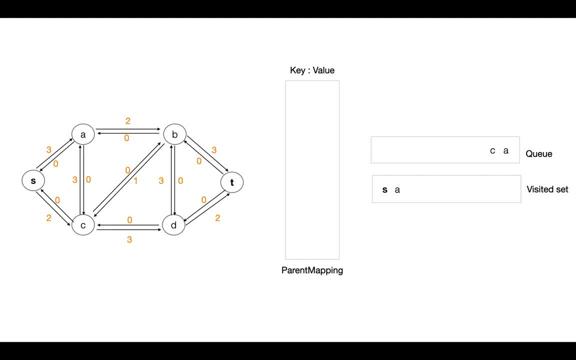 queue, and also to the visited set as we are visiting them. and now to this parent mapping with along with the mapping. so this says that we came to a through s, and we do same for the other vertex, which is c. we came to c through s. that's why it is. 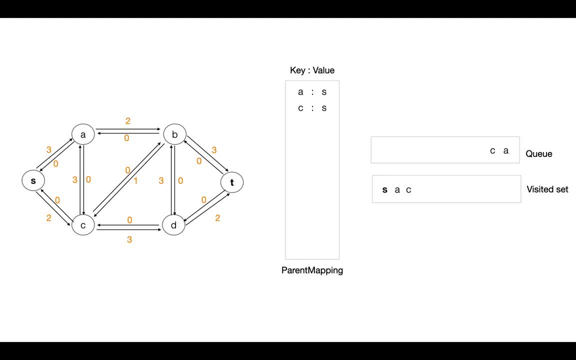 c, colon s. c is the key and the value for c is s. so now we're done for s and now we select the next vertex that we have in the queue. so next vertex that we have in the queue is a. so now we're going to look for the forward edges going outwards from this a to the other vertices. 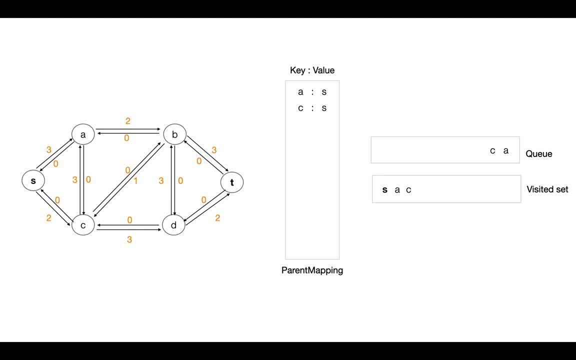 having value greater than zero and which are all not already visited. so see, there are three edges going outwards from a. these are a, s, a, c and a- b. but as s and c are already visited and also these edges are having value zero, so we are not going to select them. but this edge a b is having a. 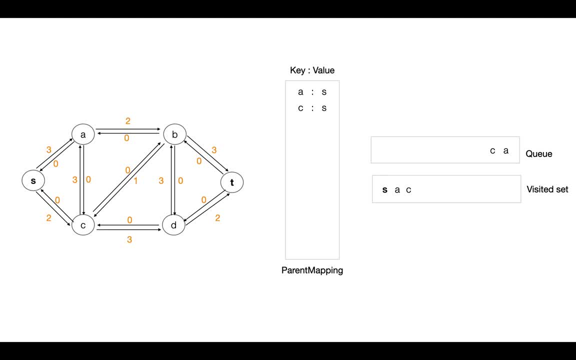 capacity two. so we're going to select this vertex b while we pull a from the q, and we're going to put b in visitor set as well. and now let's put it in the parent mapping along with the mapping as we came to b through a. now the next edge that we have in q is c, so c is also having. 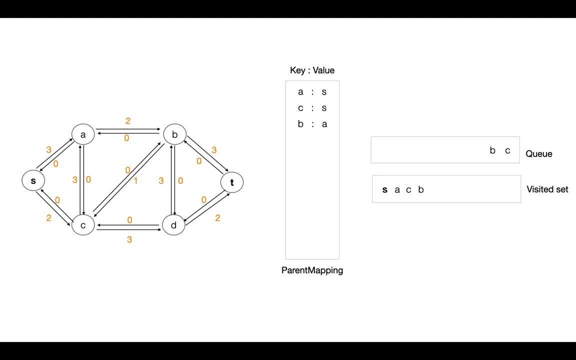 c, a, c, b and cd, these three edges, but we can only consider this last edge, cd, as it's having capacity greater than zero and it's not already visited. a and b are already visited, so they are not in the game, so let's select d, while we pull c from the q. 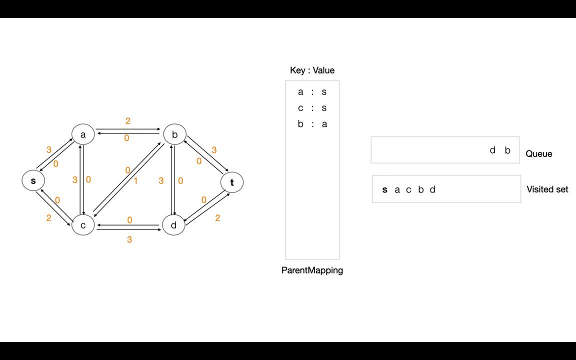 let's put in, put d in wizard set and also in plant mapping. now pull b from the queue and while we pull b we gonna put the vertices, the connected vertices, from it. so the edges that are going outwards from b are bt and bd and bc and ba. but a is already visited. c is already visited. 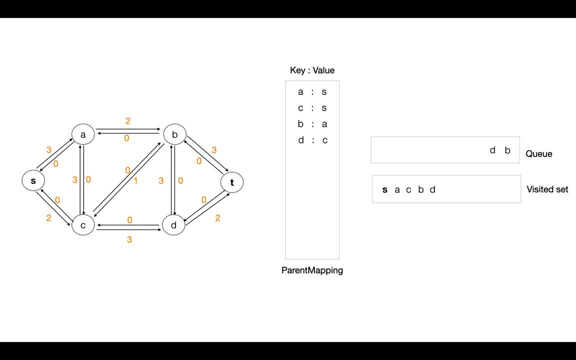 d is already visited, we are left with t, which is sync, and here the loop gonna stop. so while we pop b from the q, we add sync vertex, which is t, into the queue, and here we stop and we add this mapping to parent mapping, saying we came to t through b, so now this parent mapping. 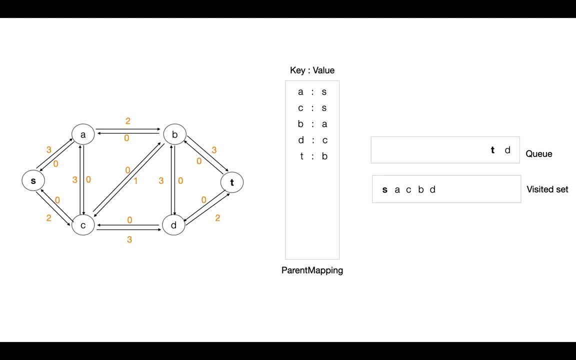 is going to help us to construct the augmenting path. we start from sync and then we go all the way to source to find out the augmenting path. so we reached to t through b and then we came to b through a and we came to a through s. so this gives us the augmenting path. now this path is from: 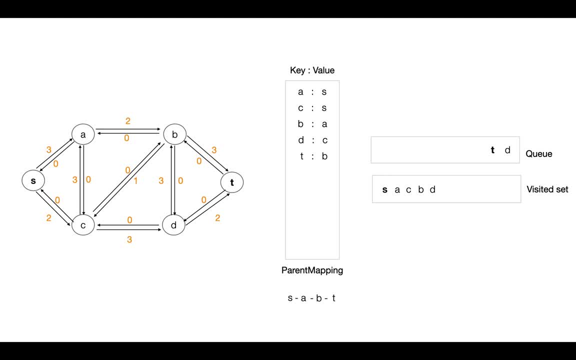 sync to source. now we reverse it to get it from source to sync. now the next step is to get the bottleneck capacity. the minimum capacity that this path is having is two. so we are going to increase the flow by two in this path. so we are going to 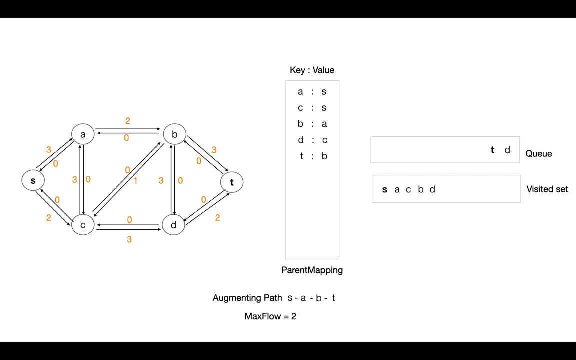 get two as the current flow for this path and also as the max flow for the complete network for now, as this is residual graph and we are increasing the flow by two in the path. so, after increasing the flow, all the shrinking capacities of this path will now have two units of water that they